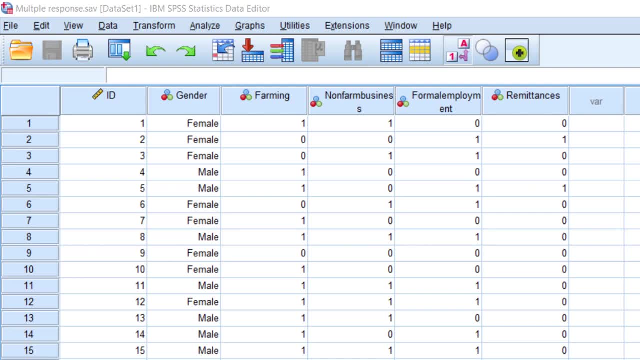 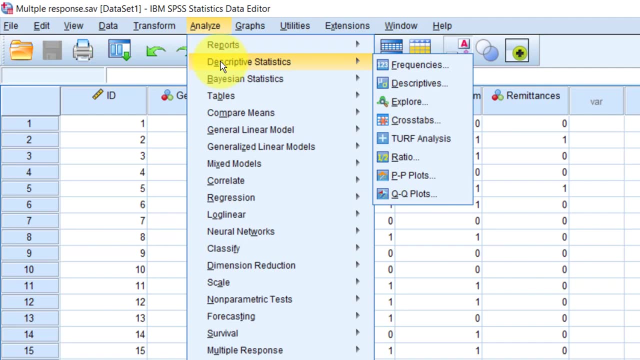 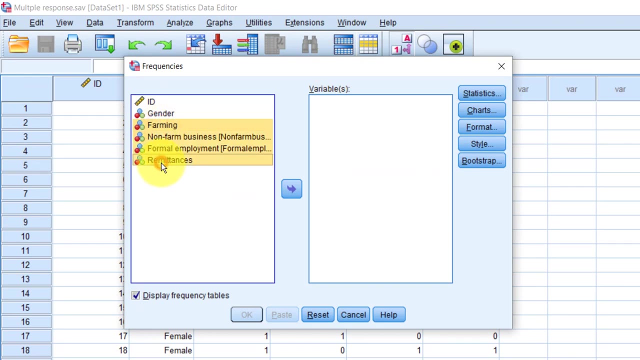 The first option for summarizing multiple response questions is to run Frequency Tables for all the variables. Let's try that. So go to Analyze Descriptive Statistics Frequencies. I'll grab all the multiple response variables, except the ID, into the variables box on the right Click OK. 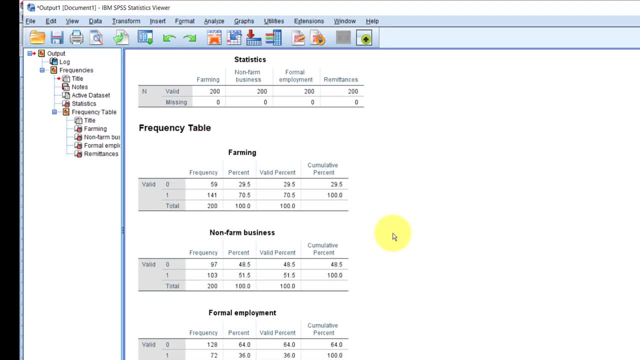 Right, the output is OK. At least from here we can tell that, for example, 70.5% have farming as one of their household sources of income. For an unfarmed business that's 51.5%, And so on. 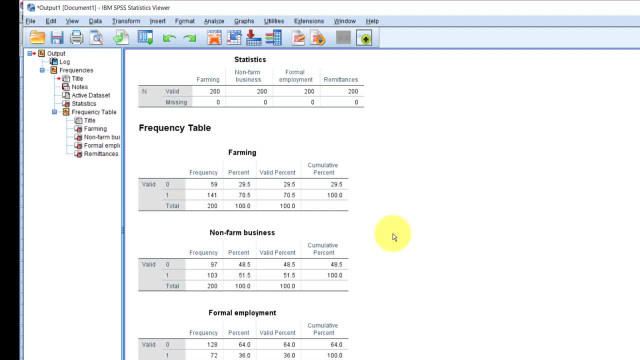 The problem with this, however, is that there are way too many tables. In most cases, we are only interested in the frequency of those who chose each of the options we have. That means we are only interested in counting the ones, and not the zeros. 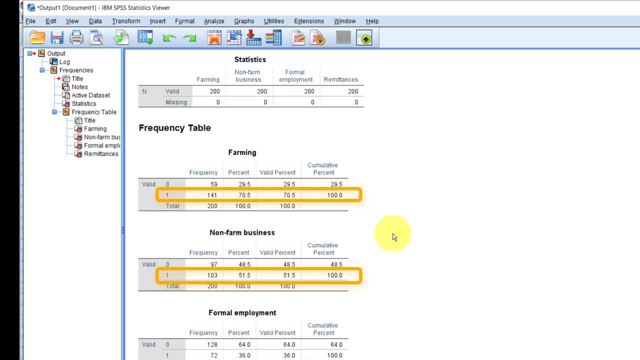 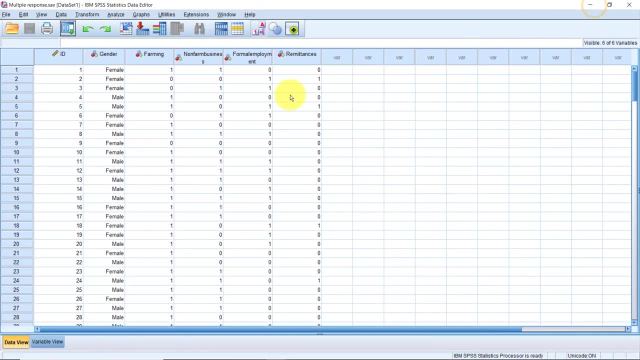 This is where you need to use multiple response options in SPSS. First, you need to define each multiple response set. Let's minimize the output. You'll find that there are several places for defining multiple response sets in SPSS, for reasons best known to the developers at IBM. 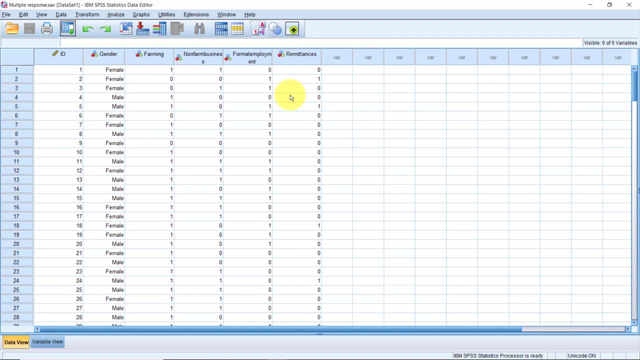 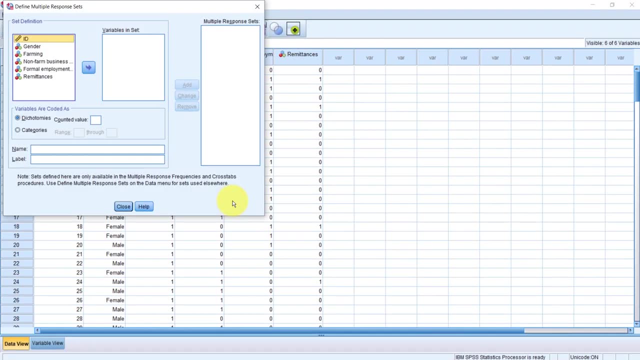 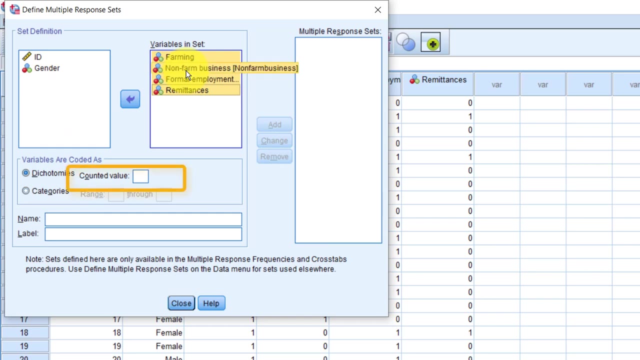 And unfortunately you need all of them. Let's start with going to Analyze Multiple Response. Define Variable Set. We'll drag all the variables in our multiple response set to the right-hand side. Then we'll specify which values we are going to be counting here, where it says Counted Value. 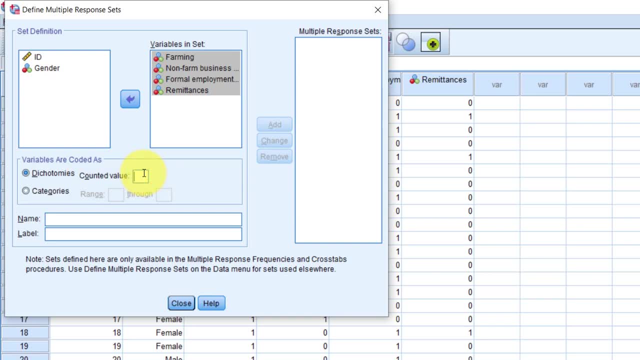 Remember that we are only interested in counting the number of people who actually selected the response, and when they did so, we recorded 1.. So we'll type 1 as the counted value. Then we need to give a name to the variable that will hold our multiple responses. 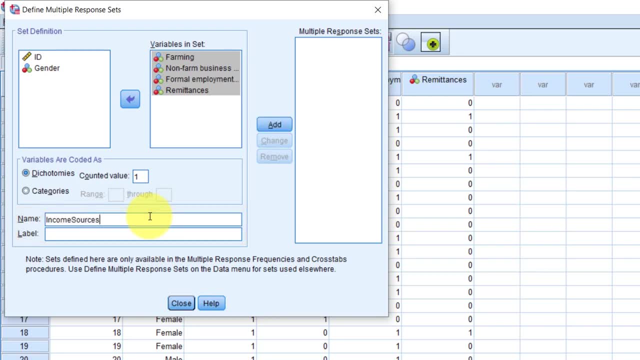 I'll say Income Sources, Without a space- remember this is a variable name- Then we can specify the label of our variable. I'll say Household Sources of Income. Then click Add. If you have more multiple response sets, you can continue in the same manner, adding the variables to the variables in the set box. 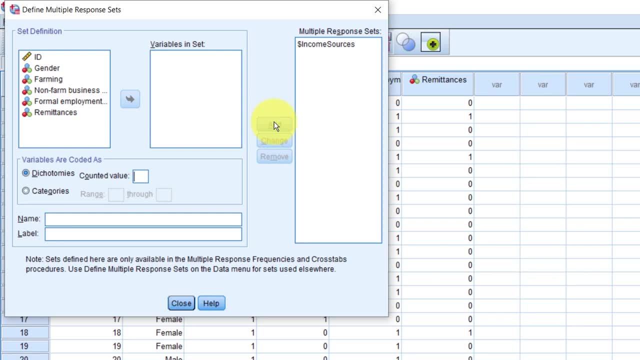 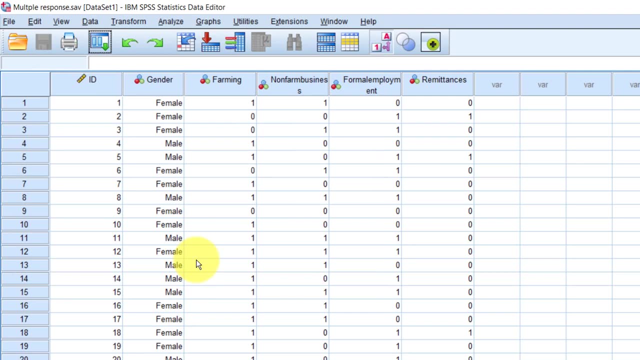 and specifying the value you are counting. Then finally, the variable label and the name. Let's close this. So, now that we have our variable, we can use it to create one table of frequencies. but we can only do that using the Multiple Response option on the menu. 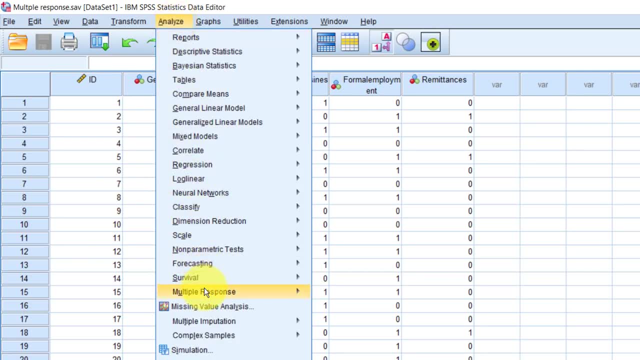 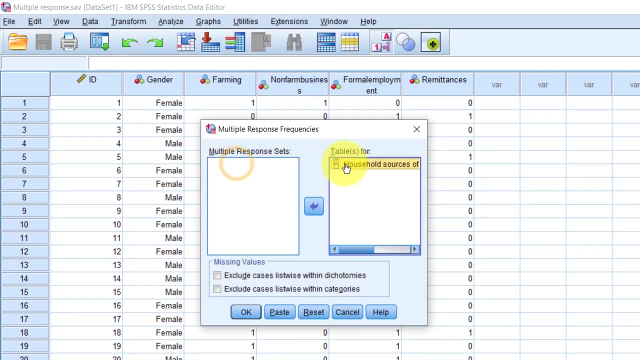 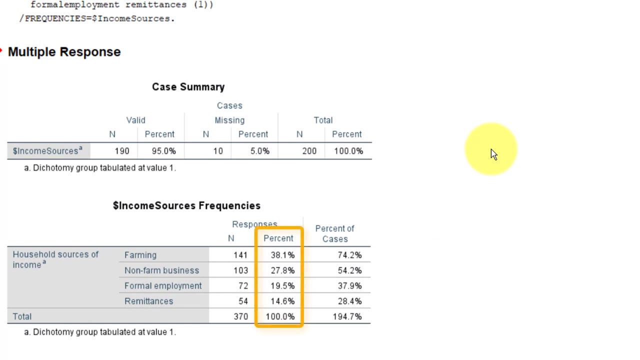 So I'll click Analyze again. Multiple Response Frequencies. Drag the Multiple Response variable to the right-hand side, Then click OK. This looks so much neater. The percent value is expressed out of the total N at the bottom. 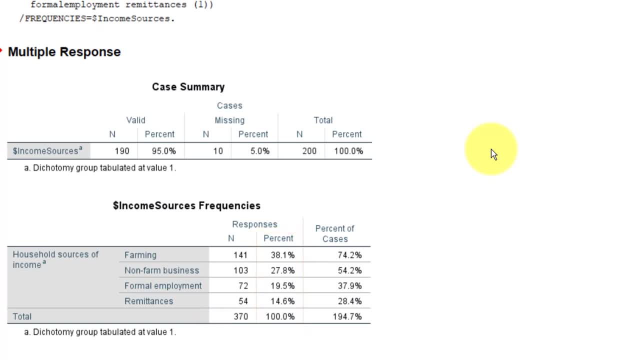 The total N here is not the number of cases in the dataset, but rather the total number of times all the options were selected combined. Since these are multiple responses, the total N is bigger than the actual number of cases, So the percent should be construed as frequency relative. 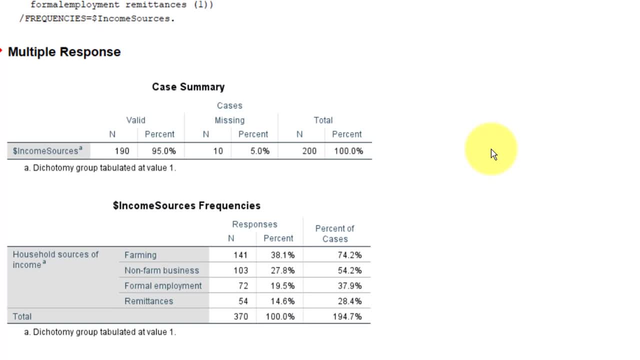 to the total number of the number of times all the options were selected, While the percent of cases here is for each of the option out of the total number of cases we have in the dataset. It's exactly the frequency we had earlier on when we used the frequency procedure. 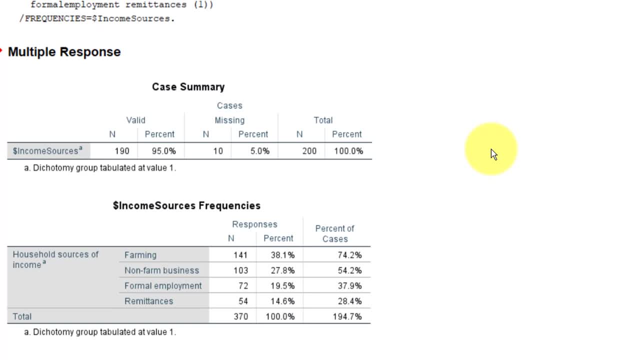 to summarize each of the variables individually. So the percent should tell you which option was selected the most out of all the options. But percent of cases should now tell you the real representation of how many times the option was selected by the total number of cases. 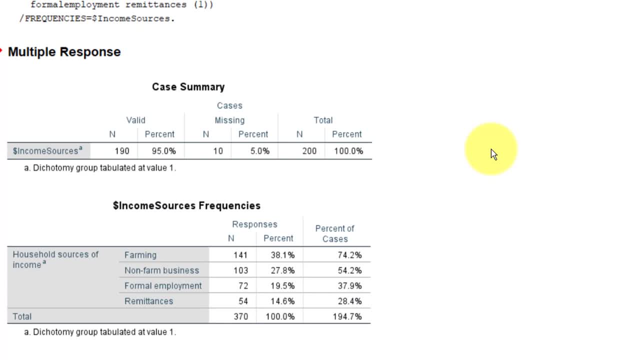 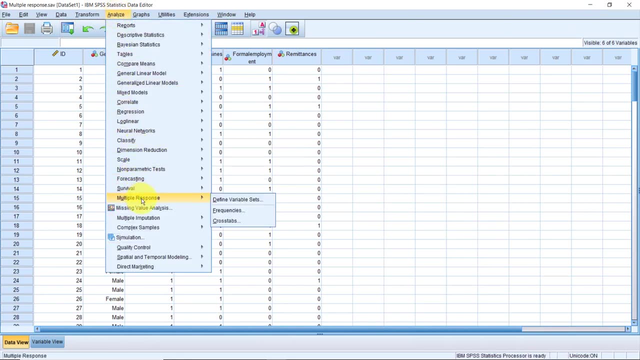 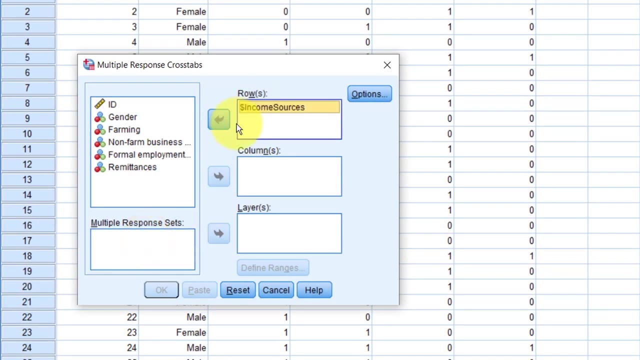 You may also have noticed that we can produce a cross-section cross-tabulation using our multiple response variable. Let's try that. Go to analyze multiple response cross-tabs. Let's drag the household sources of income variable here to the rows. Then let's use the gender variable in the columns. 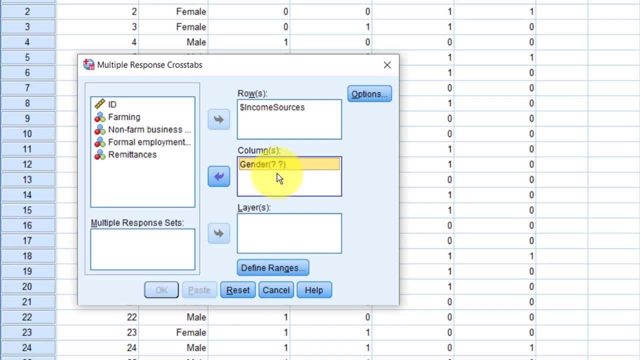 Notice we have question marks inside the gender bracket. That's because we need to specify the values of gender. So click define ranges. We are using zero for female and one for male, So we'll type those values here, Click continue. It's best to turn on column percentages. 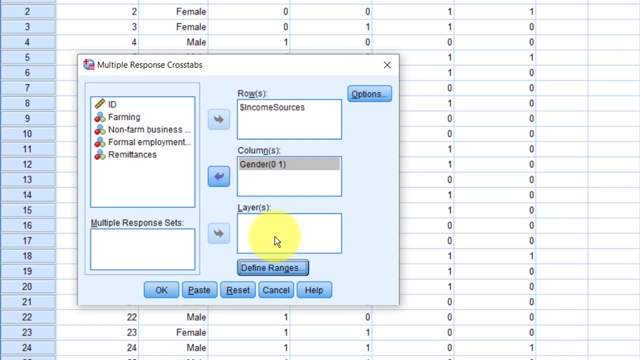 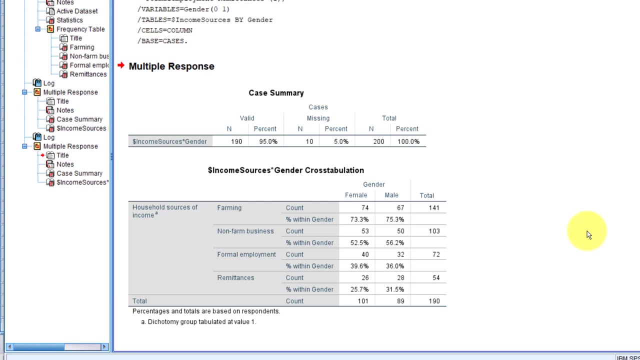 so we can see the relative frequencies by gender. To do that, click options Under cell percentages, click column, Then click continue. Finally click okay, Nice, So now each of the options has been cross-tabulated by gender, without having to worry about those who did not select the option.